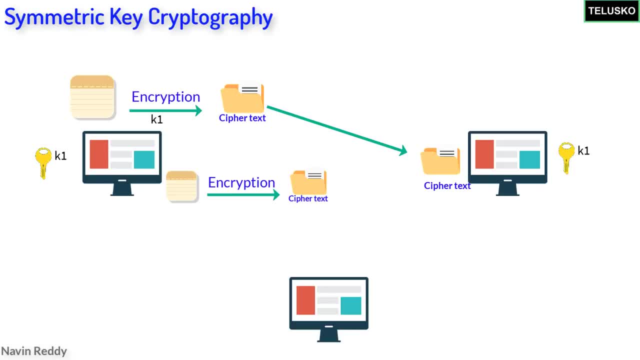 So between the A and B we have K1, between A and C we have K2.. Let's say B and C want to interact. What key they will use? Will they use K1? Of course not. Will they use? 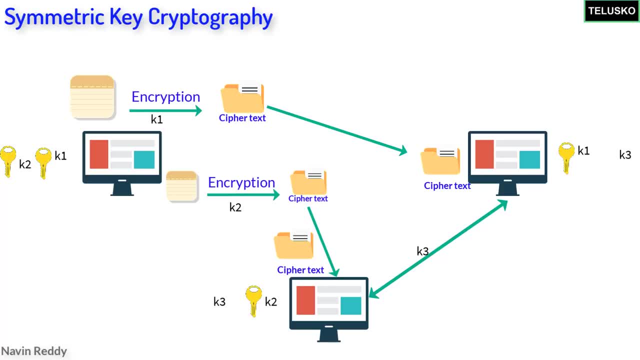 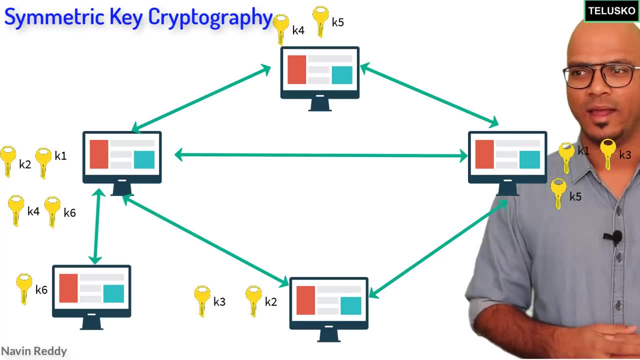 K2?? Of course not. They will need a different key, which is K3.. What I wanna say is: as the number of users increases, we have to increase the number of keys, And it will be difficult to manage, Right? So, for example, let's say we have A and B, K1,, K2.. Let's say: 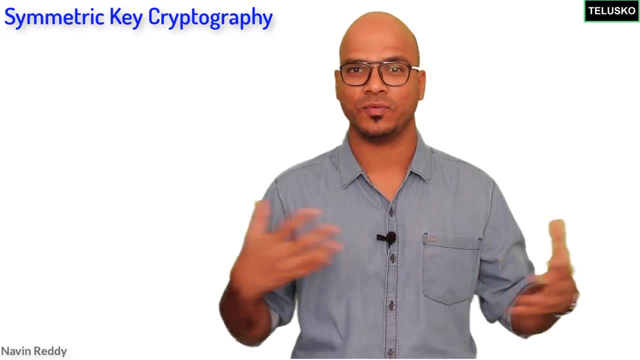 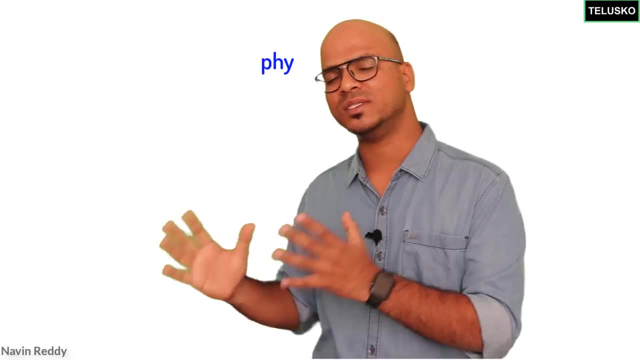 right example. in my pocket i have to carry 100 keys, because if i want to interact with 100 people, i have to manage all the keys. we don't want that. so that's one of the drawback of symmetric. let's move towards asymmetric. asymmetric cryptography, also known as public key cryptography. 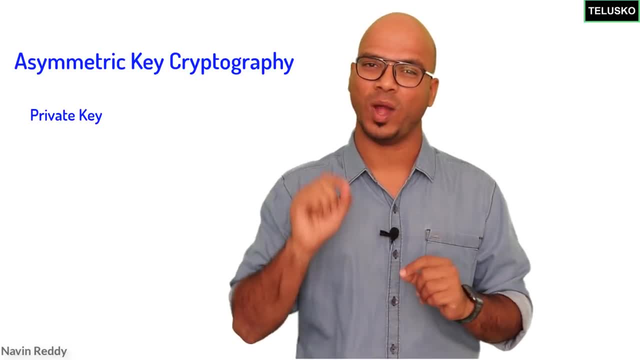 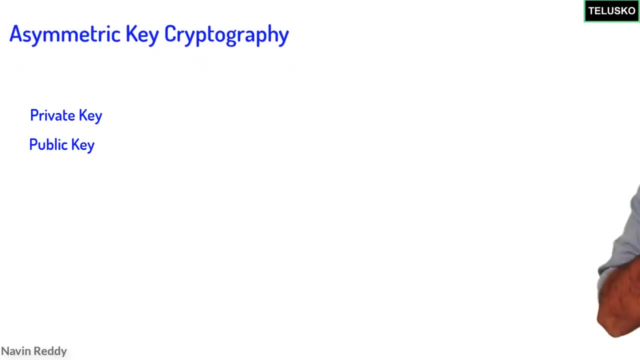 so basically we use two different keys here. one is private key and one is public key. so what is this? public key and private key? as name suggests, everyone will have two keys. let's say: a- want to send a message to b. b- send a message to cs. so on this network we have multiple nodes. 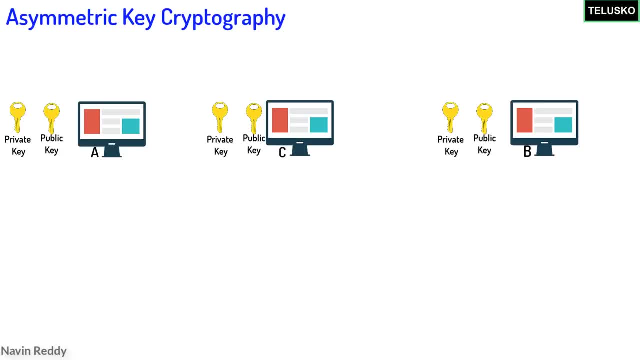 each node will have two keys: the private key and a public key. so a will have its own private can public key, b will have its own private and public key. c will have its own private can public key. if you want to encrypt and decrypt the message, you have to use both the keys, not one. so to encrypt a. 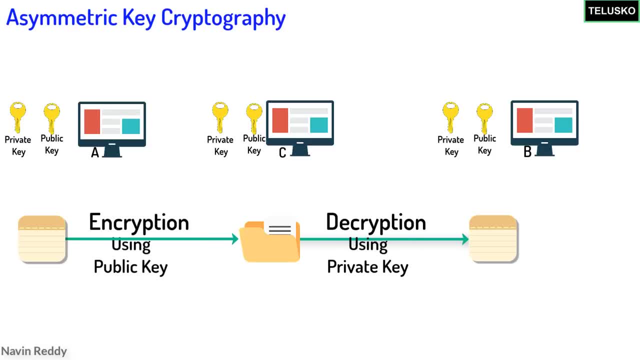 message. you can use public key, but to decrypt the message you have to use private key. if you are using a private key to encrypt the message, then you have to use a public key to decrypt a message. so you have to use both the key at the same time. You can't simply say: I will encrypt with public key and decrypt. 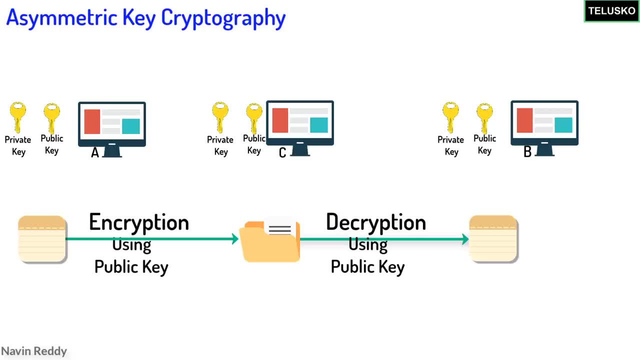 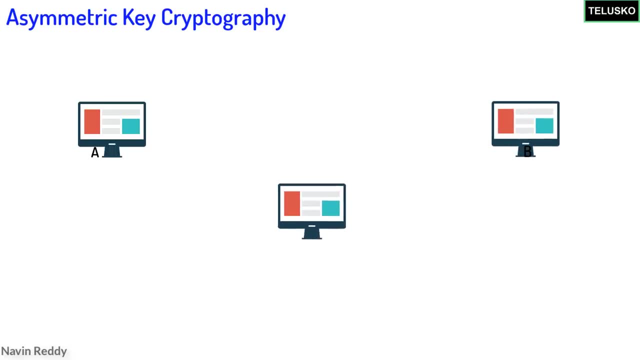 with public key. That's not possible, So we have to use both. So if you are encrypting with private, you have to decrypt with public key. If you are encrypting with public, you have to decrypt with private. How do you achieve security here? So let's say, if A want to send a message to B. 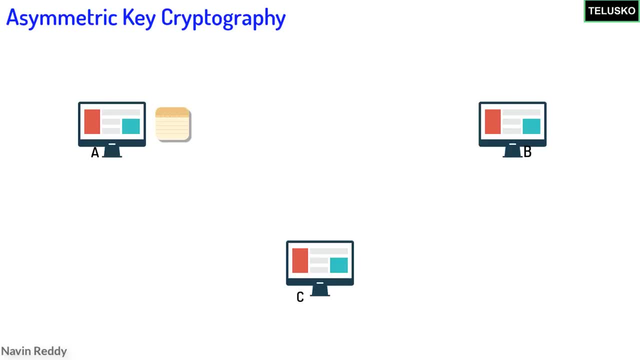 As we know, the public key of B is known to everyone- Public right- So of course A will also know the public key of B. So what A will do? A will encrypt the message with B's public key and then that message goes to B. Of course everyone else on the network can see that message. 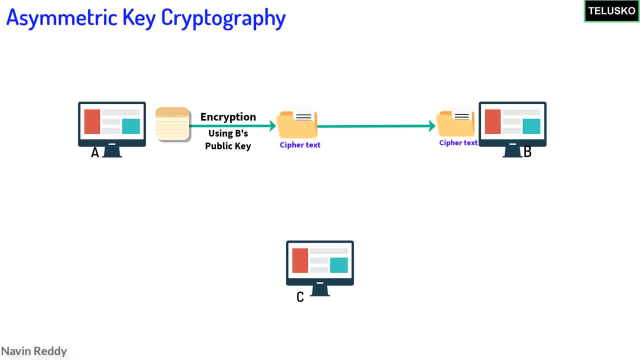 the encrypted message, but no one can decrypt it. You know why? Because that message will be decrypted only with B's private key. and who has B's private key? Of course only B, the private right. So you will know your private key and everyone else will know your public key. So that's how you do it. 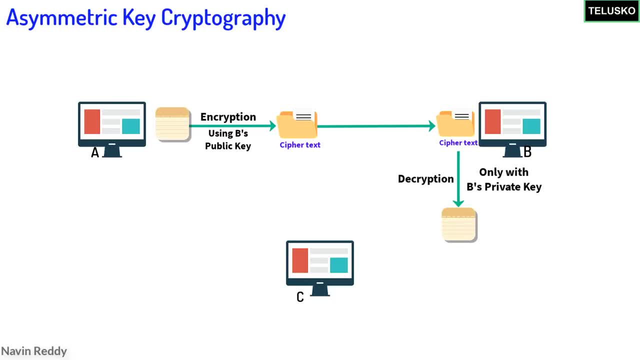 So how to achieve security: Encrypt the message with public key and decrypt the message with private key. Let's do it Again. so let's say C want to send a message to D, So which public key C will use? So C will use a. 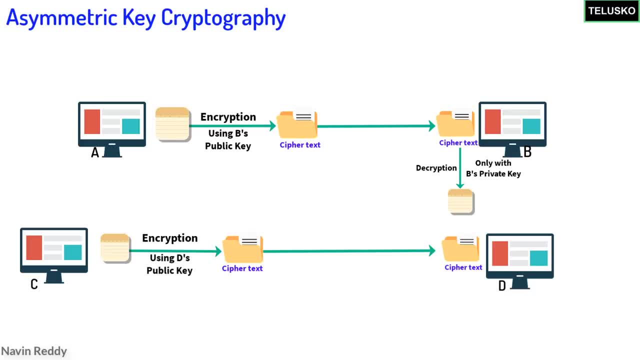 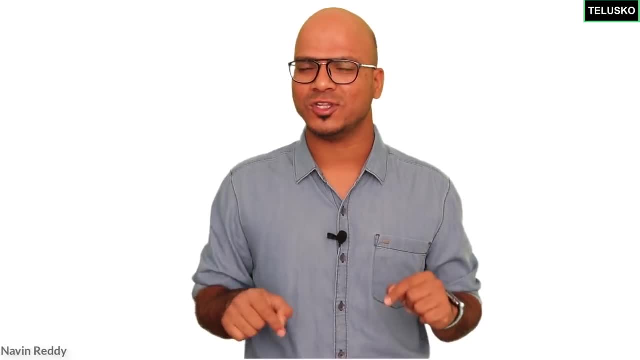 public key of D. So C will encrypt the message with D's public key and D will decrypt the message with its own private key. So that's how this cryptography works. But now the question is: what is that key is? Is it a number? Is it a text? That we'll discuss in a separate video. We'll 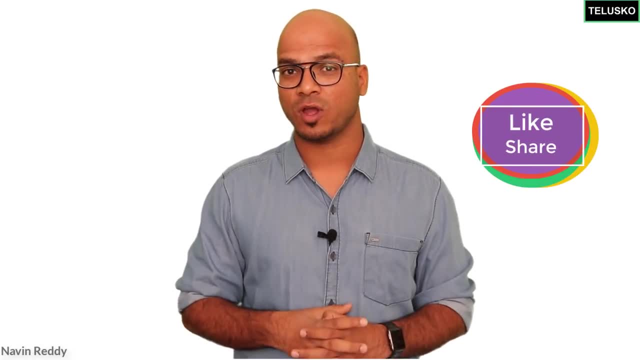 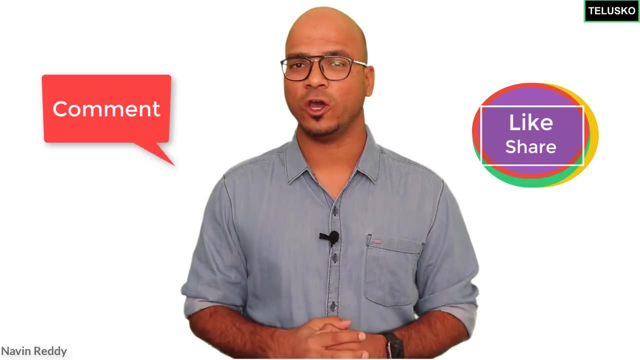 talk about how exactly to get a key. So that's it from this video, where we have talked about types of cryptography. In blockchain, we'll be using the public key cryptography. So, yeah, that's it from this video. I hope you enjoyed it. Let me know in the comment section. and do subscribe if you have not done yet. Bye, bye. 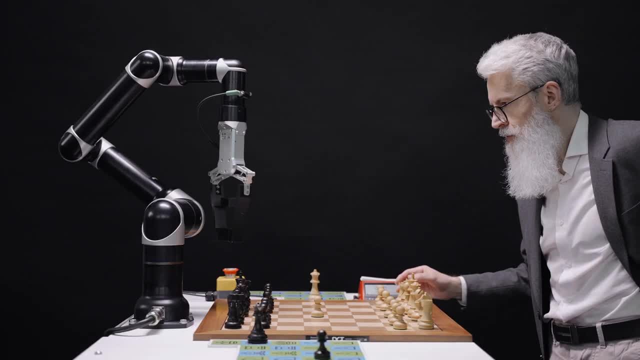 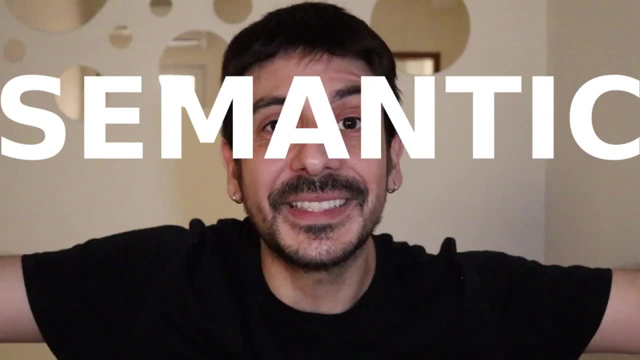 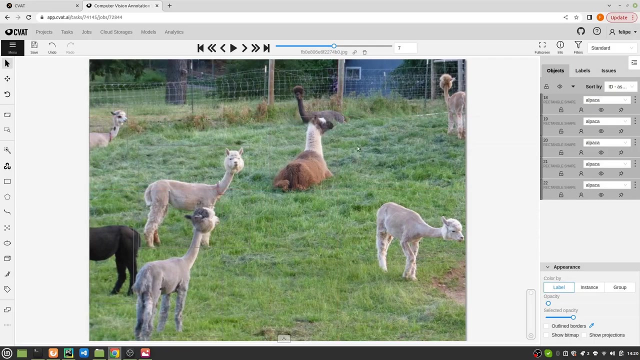 YOLOv8, one of the most powerful computer vision technologies ever made. In this video, I'm going to show you how to do object detection, image classification, image segmentation and pose detection on your own custom data using YOLOv8.. I'm going to show you the entire process. 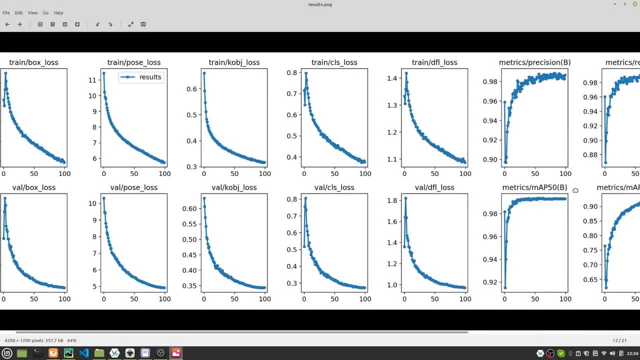 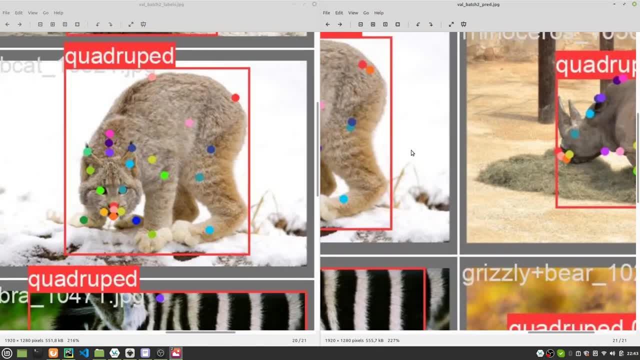 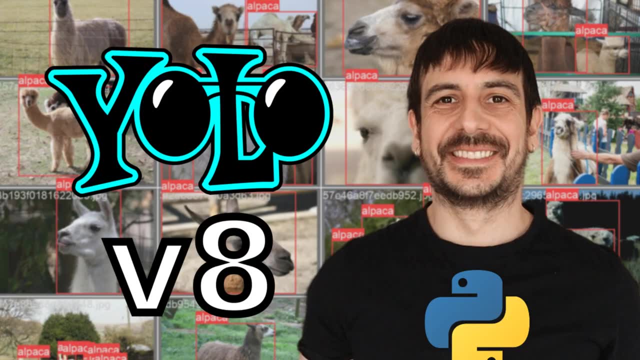 how to annotate your data, how to do the training, how to analyze the performance of the model you trained and how to use the model to make predictions. This is a full, comprehensive tutorial on YOLOv8, and now let's get started. Hey, my name is Felipe and welcome to my channel. 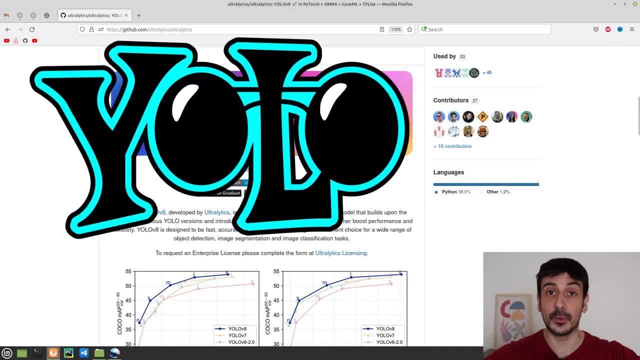 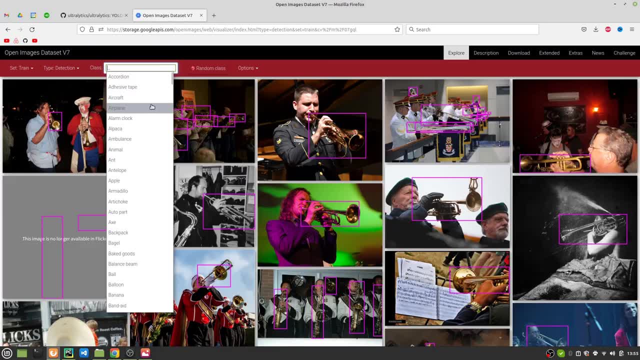 In this video, we are going to train an object detector using YOLOv8, and I am going to walk you step by step through the entire process: from how to collect the data you need in order to train an object detector, how to annotate the data using a computer vision.